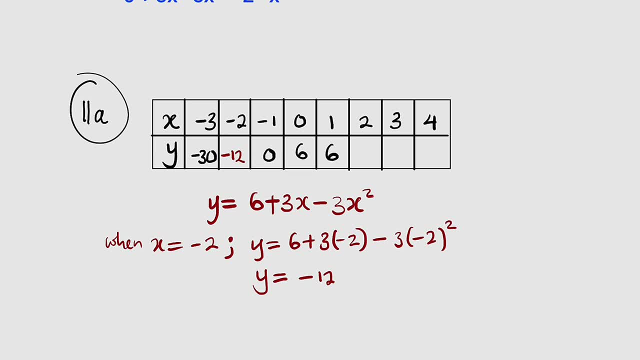 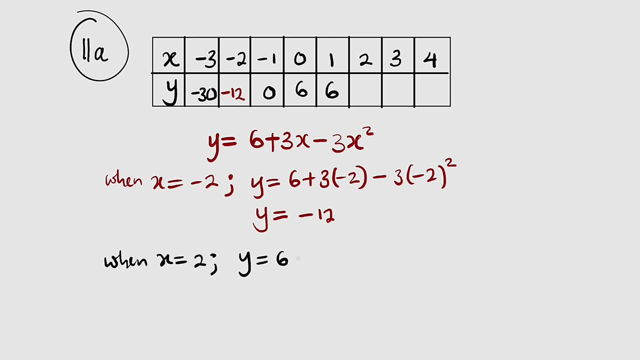 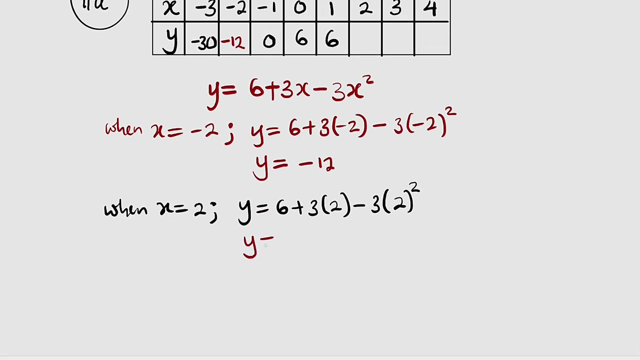 here Already, these three are given. Then let's jump to when x is 2.. We have y equal to 6 plus 3 multiplied by 2 minus 3 multiplied by 2 squared. If you simplify this, you're going to obtain the value of y to be equal to 0, which implies that we have 0 right here. 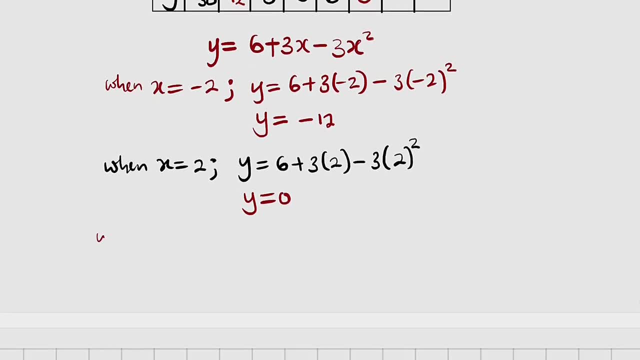 Moving on, When x is equal to 3, we have y equal to 6 plus 3, multiplied by 3 minus 3, melted, explained by 3 all squared. If you simplify this, you're going to obtain the value of y equal to negative 12.. So we have negative 12 right here. Then the last one is when x is equal to negative 2.. 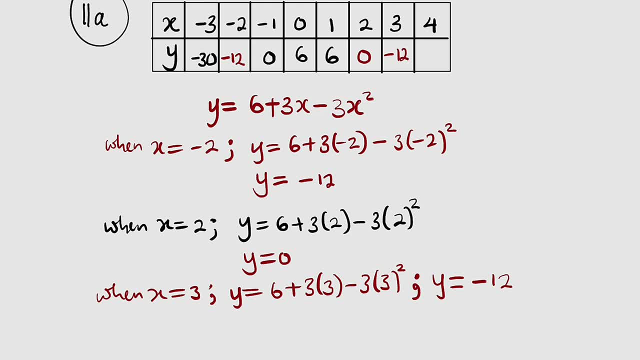 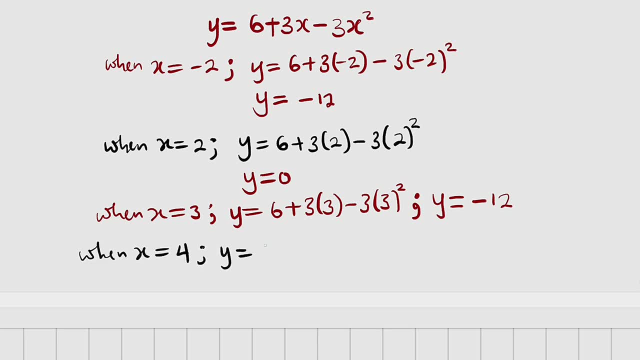 So we have negative 12 right here, The to 4.. We have y equal to 6 plus 3 multiplied by 4 minus 3 multiplied by 4 all squared. If you simplify this, you're going to obtain the value of y equal to negative 30.. So we 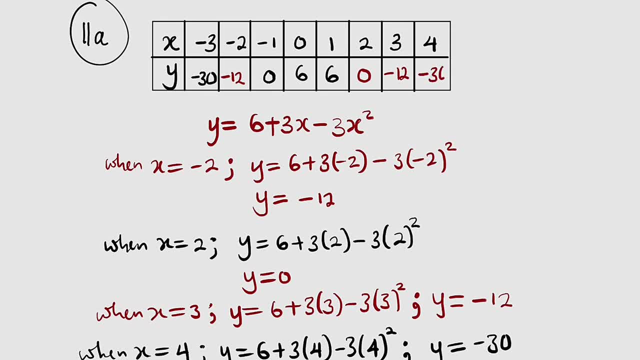 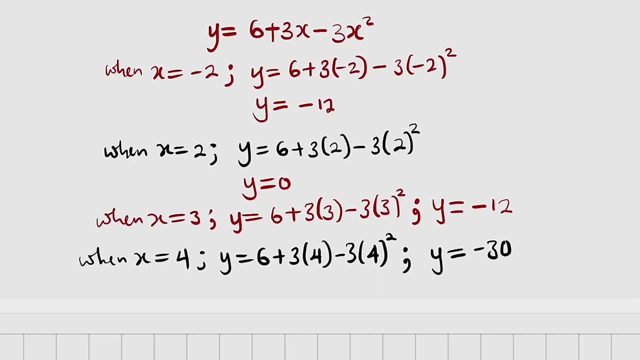 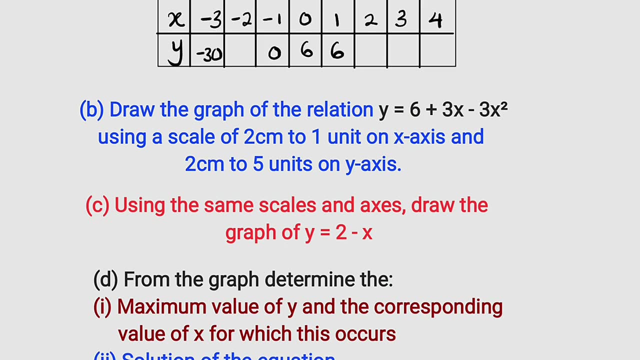 have negative 30 right here. So this is all about a part. We have copied and completed the table and you have to show this walking for you to earn extra marks. So the b part. The b part stated that we should draw a graph of this relation: y equal to 6 plus 3, x minus. 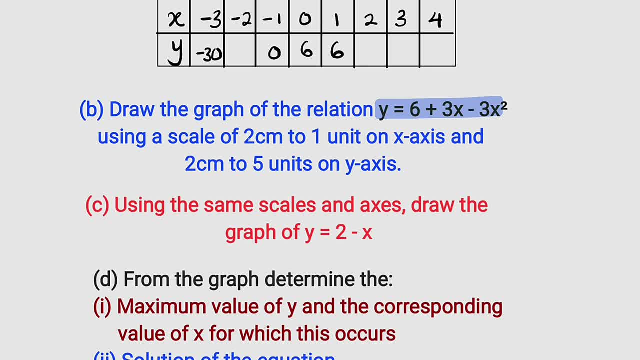 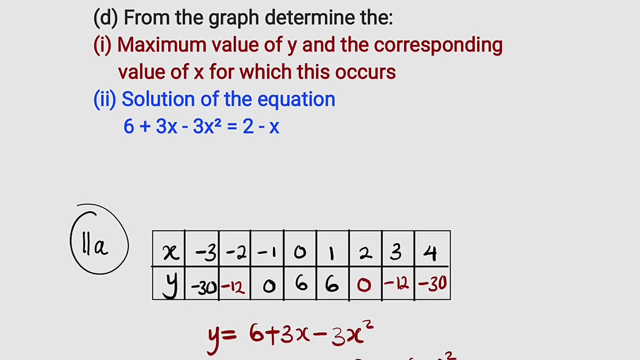 3 x squared, using the scale 2 centimeters to represent one unit on x axis and 2 centimeters to represent 5 units on y axis. So the b part. We're going to do everything on the graph sheet Already. I have planned everything. Let me just explain It. 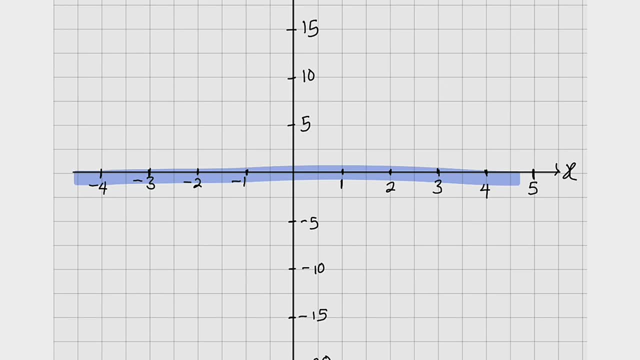 stated that on x axis, which is this, one every 2 centimeters should represent one unit. This is why you can see from origin: every box here represents 1 centimeters. 1 centimeter, 1 centimeter, 2 centimeter. I have one unit. 1 centimeter, 2 centimeter. I have another. 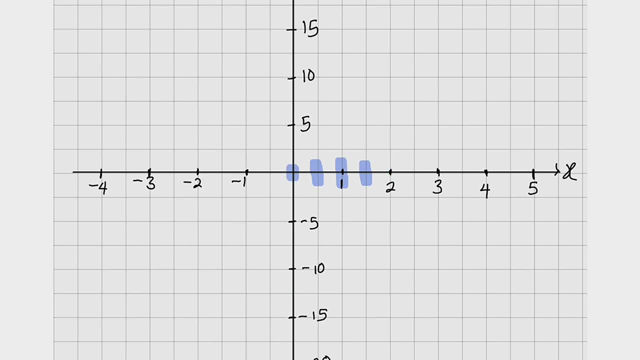 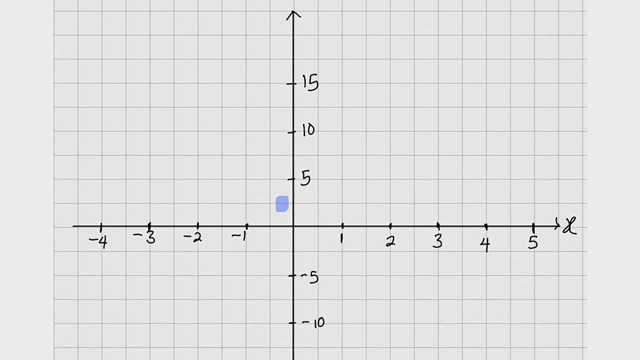 unit. This is how it is across x axis And it stated that on the y axis every 2 centimeters should represent 5 units. You can see: 1 centimeter, 2 centimeter, We have 5,. 1, 2, we have 10,. 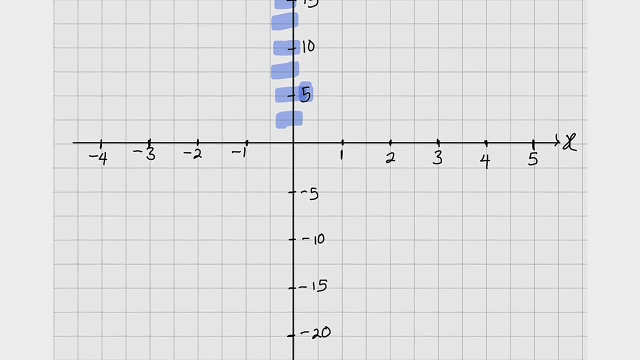 1, 2, 15,, 20,, 25,, 30. And if you come to the negative direction, you can see you have negative 5, negative 10, 15,, 20,, 25, 30.. 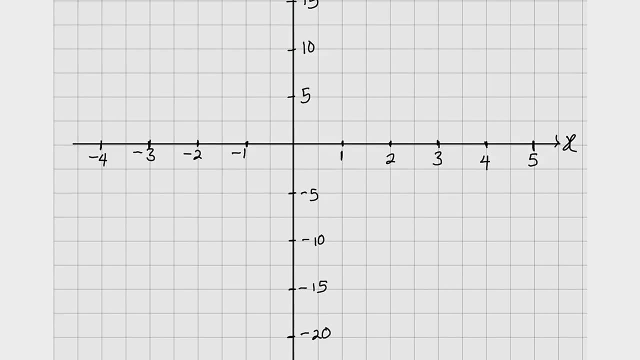 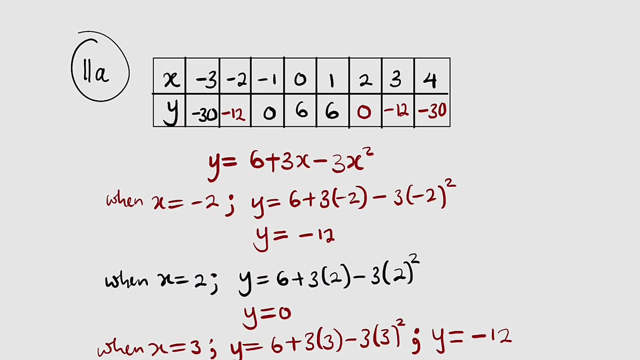 All negative values. So how can we plot a graph? To plot this graph, we're going to use our table. right here On the table, you can see the extreme end We have when x is equal to negative 3,, the value of y is equal to negative 30.. So that's what we are going to. 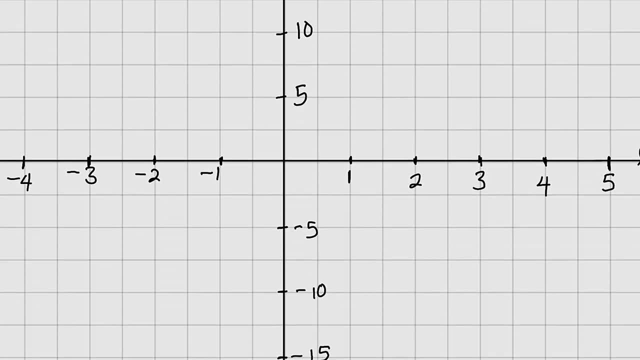 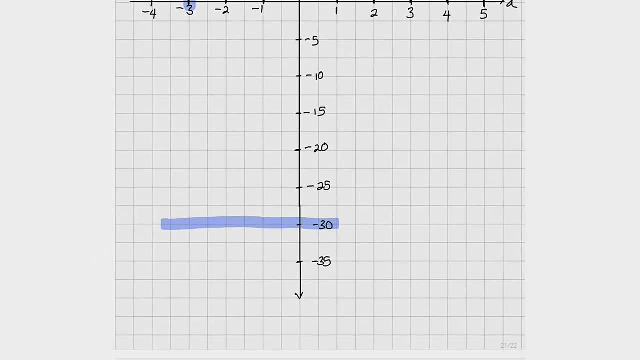 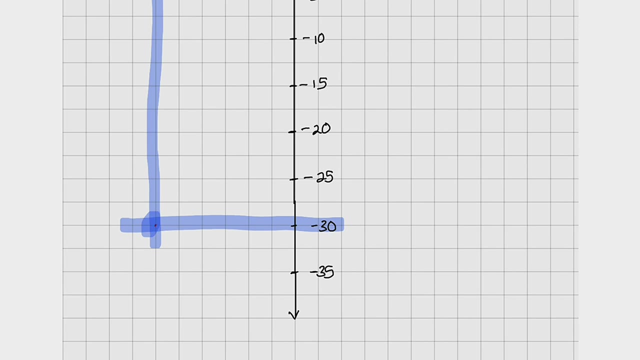 locate on the graph You can see to the left hand side, this is where we have negative 3.. And if you come down here, this is where we have negative 30. So if you come across like this, you see the intersection here. So we have 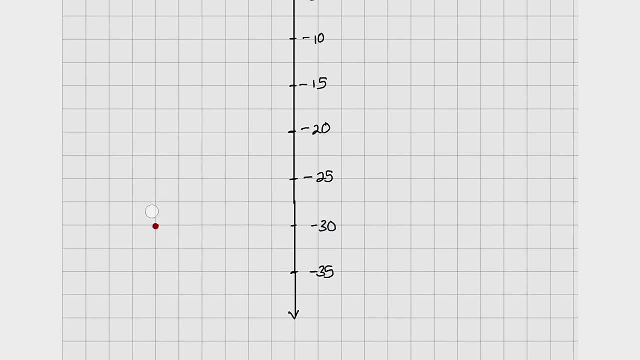 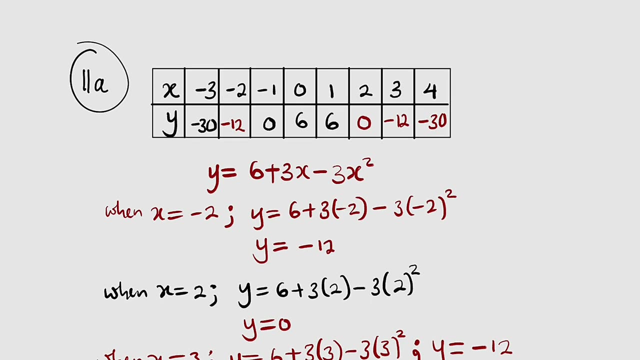 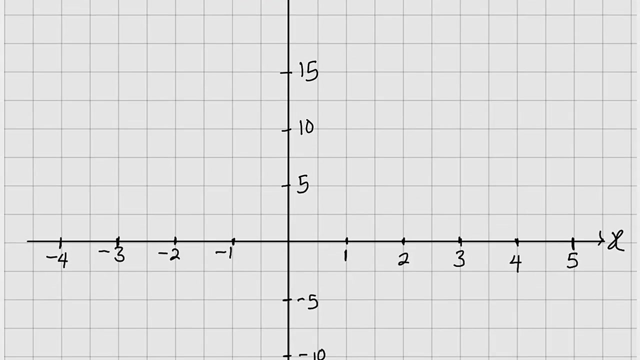 a star right here. So I'm going to clean all this. It is not necessary. And you go back again. You check when x is negative 2.. We have y equal to negative 12. So let's locate negative 2.. This is negative 2,. right, We are looking. 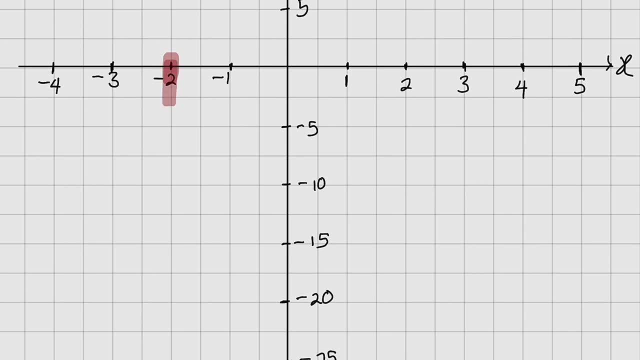 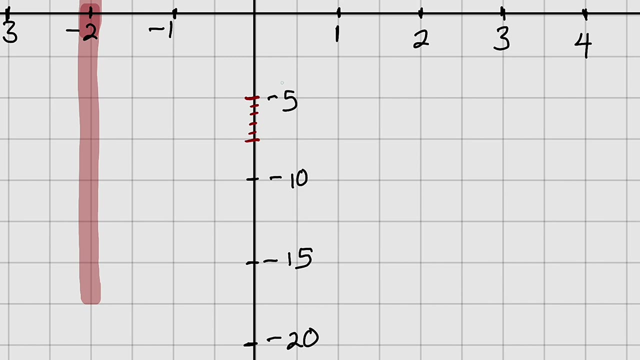 for negative 12 as the value of y. So let me take this down a little bit. You know this is negative 10.. We are looking for negative 12.. But what you should remember is that between this line to this line we have 5 extra lines, right. So between negative 5 down to negative. 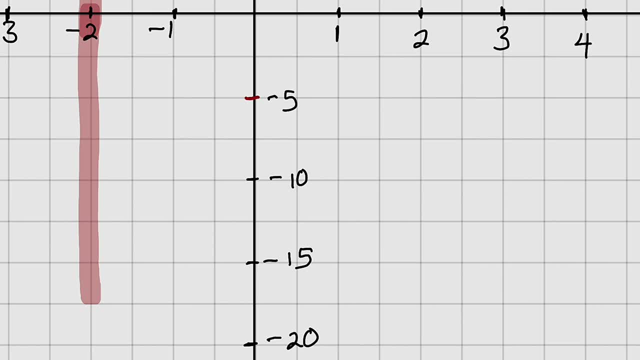 10, we have 10 extra lines, And between negative 10 down to negative 15, we have another line. We have another 10 extra small lines, So we are going to count 2, 2 to represent 1 unit. 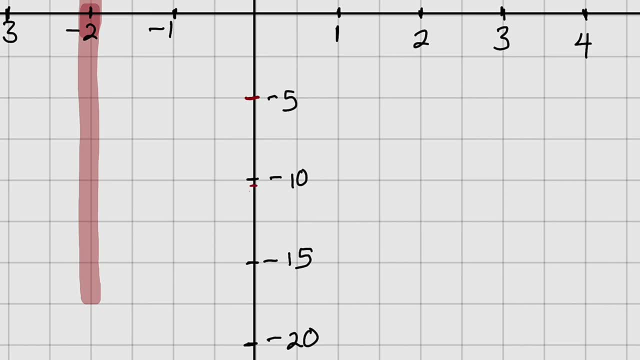 So if this is 10, we have 1,, 2,, 11,, 1,, 2,, 12.. So we have 1,, 2,, 13.. But we are looking for 12.. So we are going to use this one right here, right? So we are going to have a star. 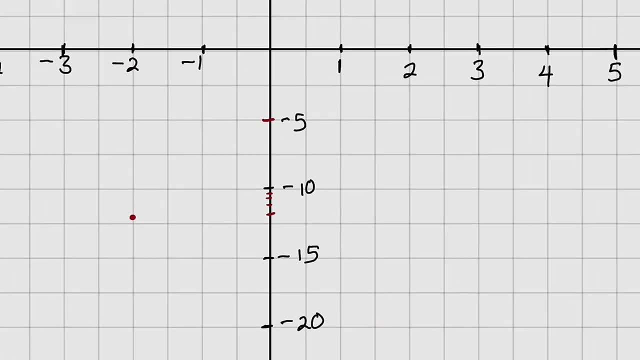 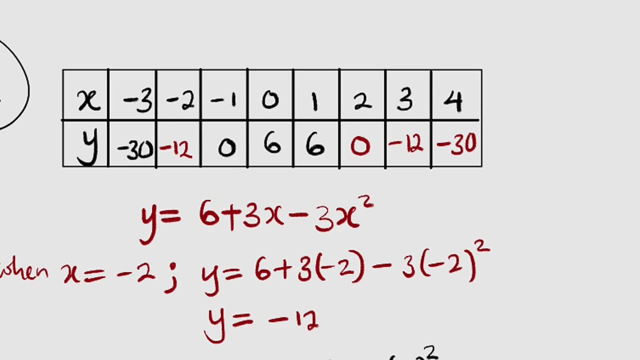 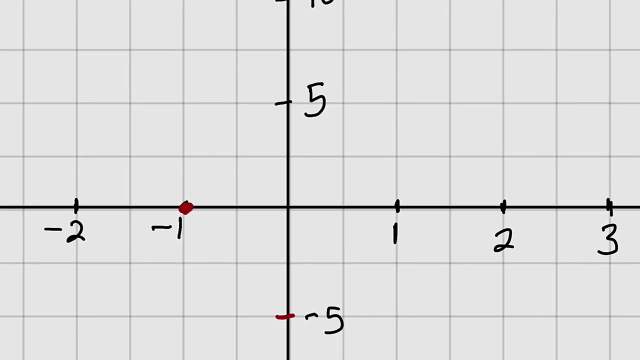 right here. Let's continue reading. Then at negative 1, at negative 1, y is exactly 0. So we are going to place a star on top of negative 1 right here. Can you see that? Then at 0, what? 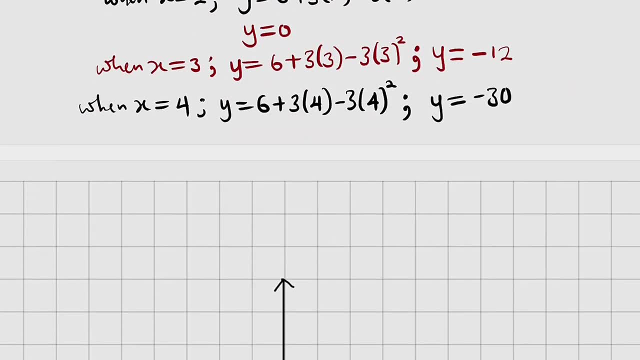 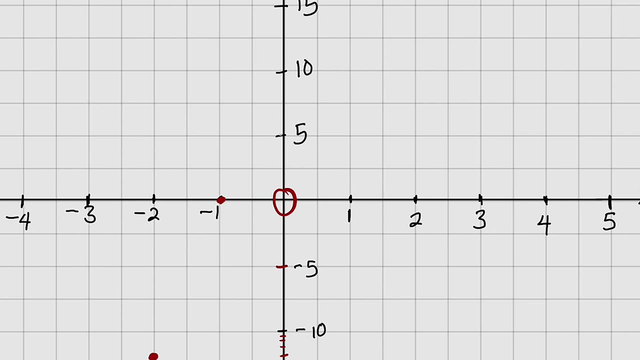 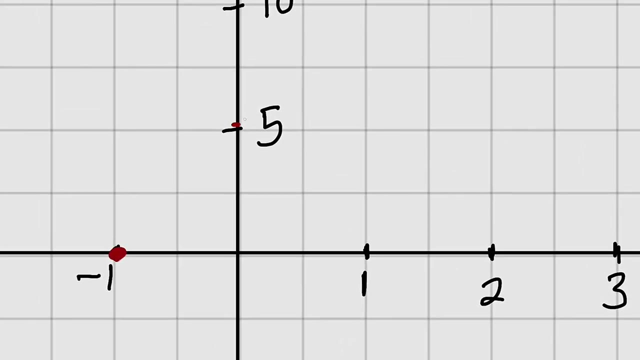 happens. When x is 0, y is 6.. When x is 0,, this is exactly where x is 0. So we are going to count 6.. Already, this is 5.. We only need to count 2 extra small lines. So if you count, we have 1,, 2, right. So let. 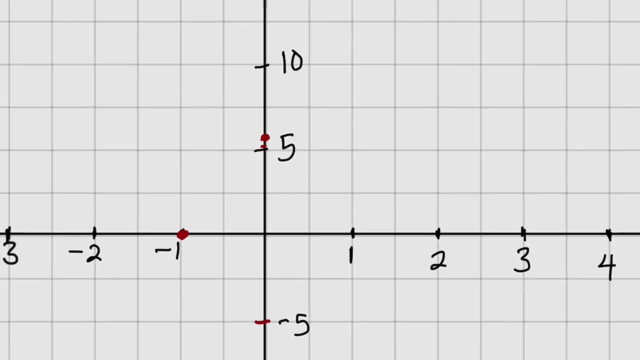 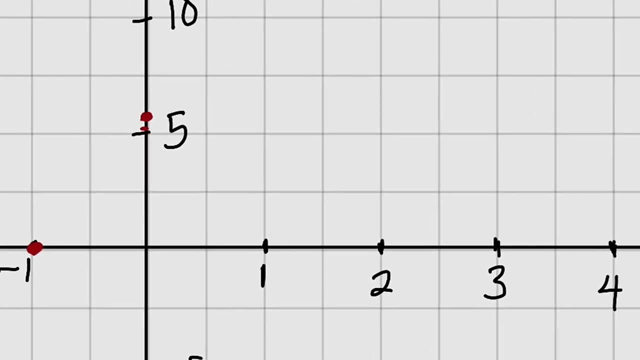 me place a star right here. Now, what happens when x is equal to 1?? It is also equal to 6 in the same direction. So we have another star right here. What happens when x is equal to 2 and y is equal to 8?? 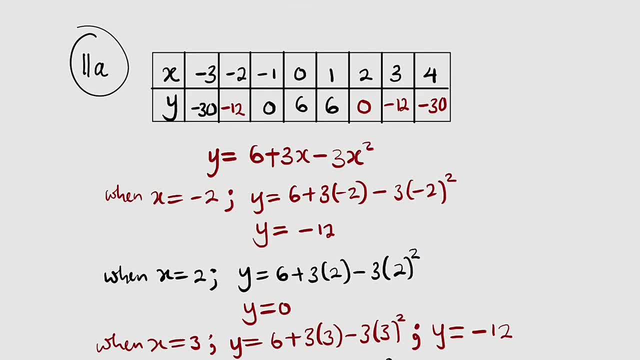 So x is equal to 2.. B, power is equal to 4.. biz tou c equals to 7.. The Pythagoreanική f equals to 10.. 9 equals to 6.. y equals to 12.. 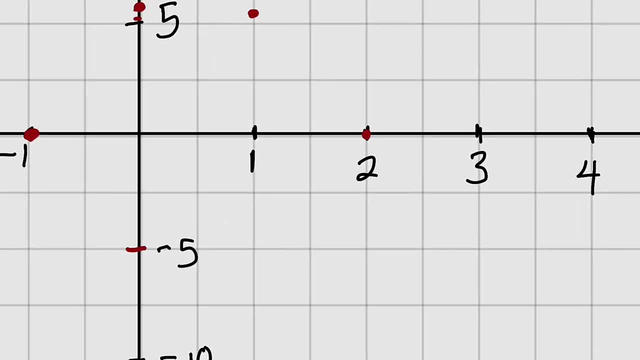 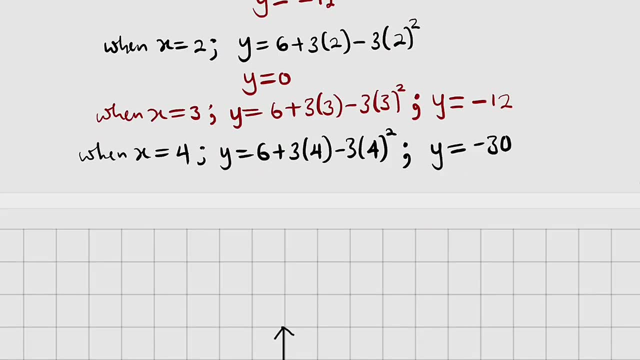 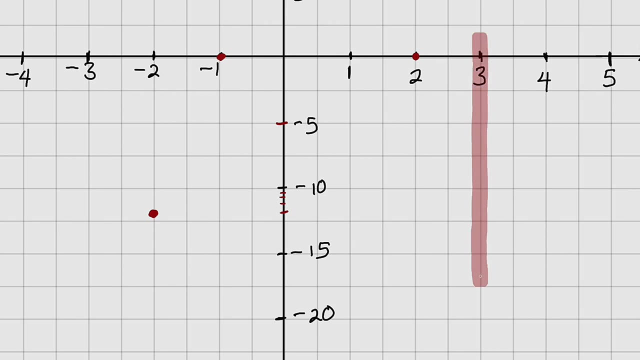 and Q equals to 5. Y equals to 2. zero. So on top of two, we have a star here. Second to the last one: when x is 3, we have negative 12.. When x is 3, we have negative 12.. Let me take it down here. Remember this: 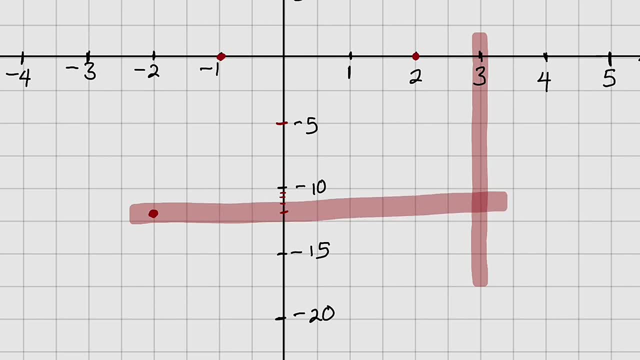 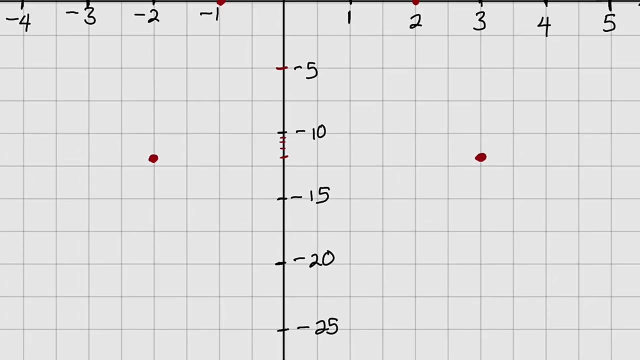 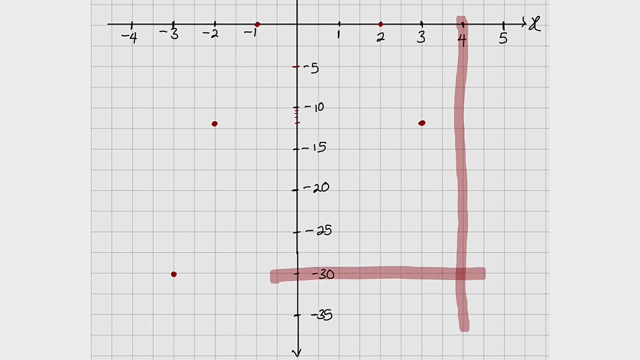 is negative 12, so you can come directly here to locate a star. So it will be somewhere here. Then the last one, when x is 4, y is negative 30. This is where x is 4, you come down to negative 30. This is where we have negative 30. So let me place a star, right? 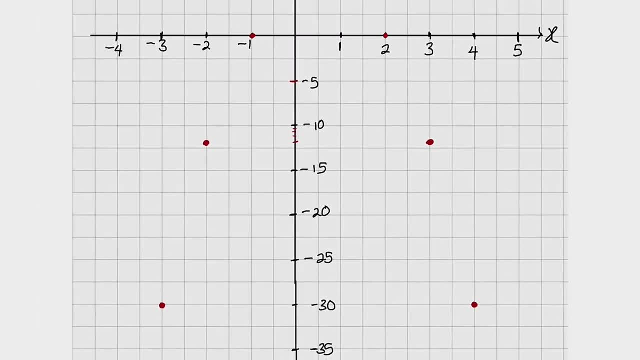 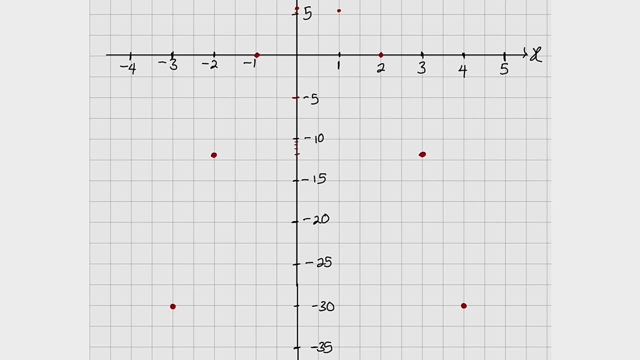 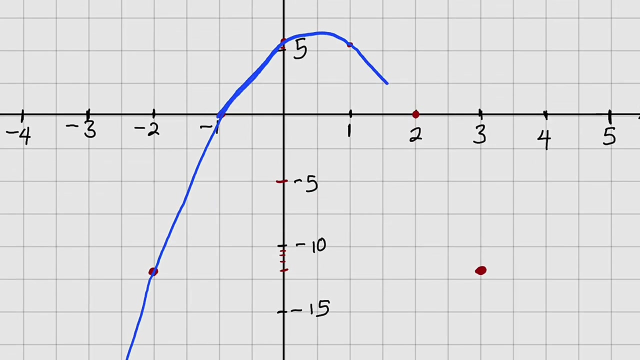 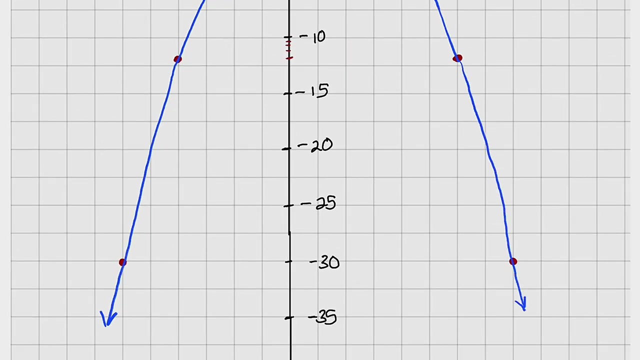 here. All right, we have just finished locating the points. What is next? We are going to join all these points in a curve direction, So let me begin. All right, you can see I have connected all the points and this is how the graph will. 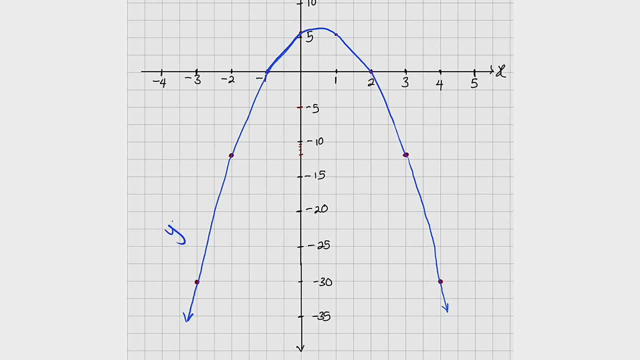 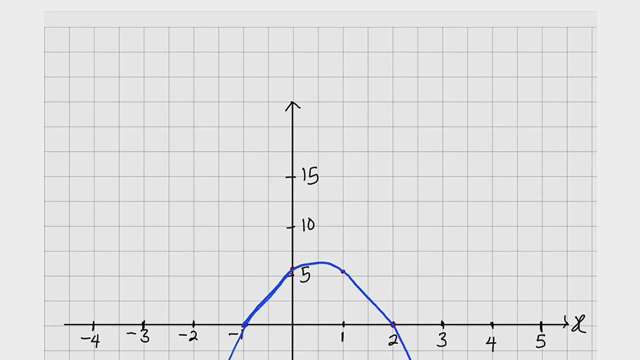 look like. So you can name the graph as y equal to 6 plus 3x minus 3x squared. Next you write the scale. We are stuck here. What? Here we are Now. it is going to take us to the bottom. what we have just now, up to there. 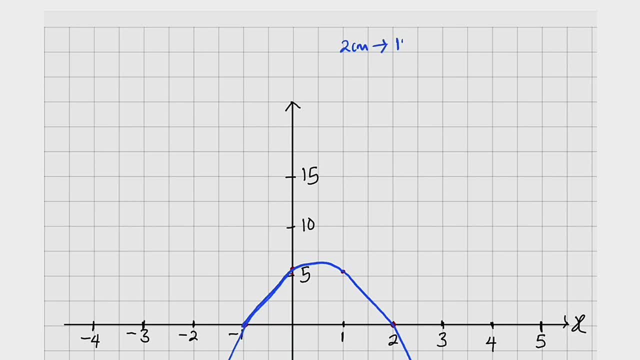 So here after you, now you remove the y and remove the negative 12.. Here is negative 18 plus 3x. You will get negative 12.. You will get negative 17, plus. remind yourself that negative 19 is minus 12, right. 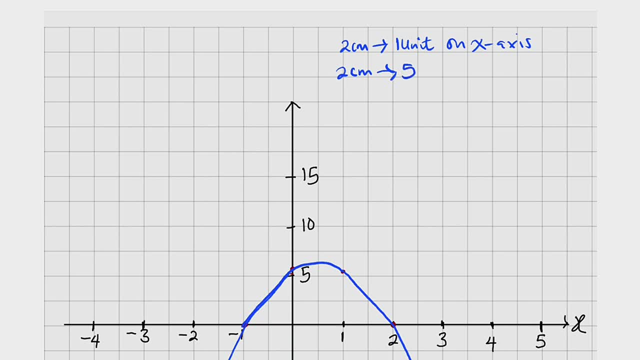 Negative〝ate TF, see if you want to stop the curve like that. So we have negative: 12 minus 3x minus 3x. negative 17 plus 3.. Negative: 20 plus 2x minus 3x minus 3x. 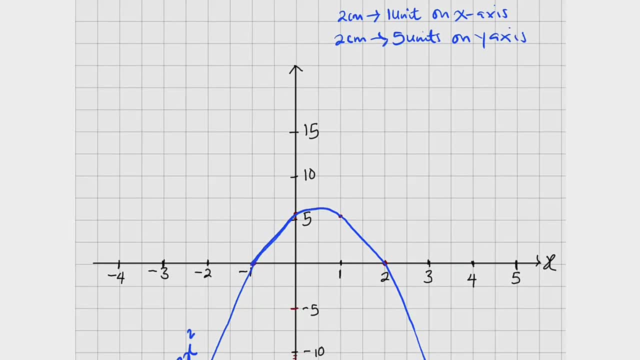 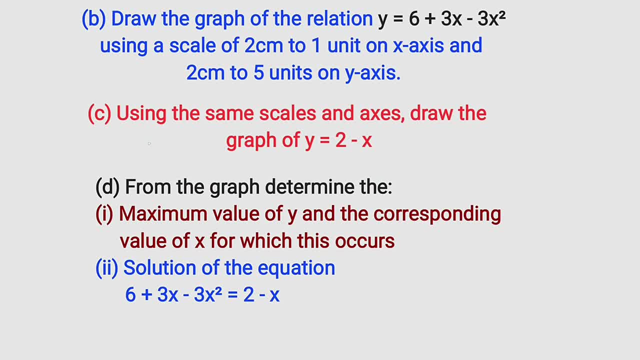 Let us move on to 11c. 11c stated that, using the same scales and axes, draw a graph of y equal to 2 minus x. This is just a linear graph, which is a straight line graph. We are going to draw it on the same graph. 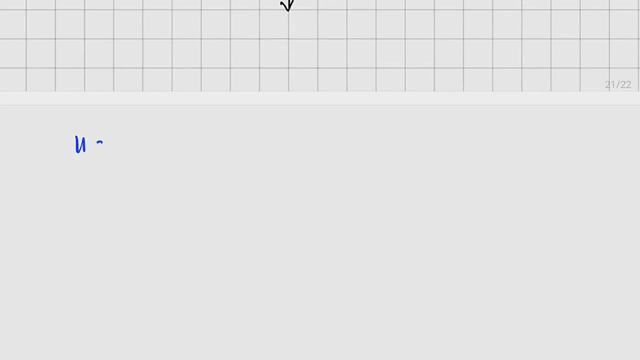 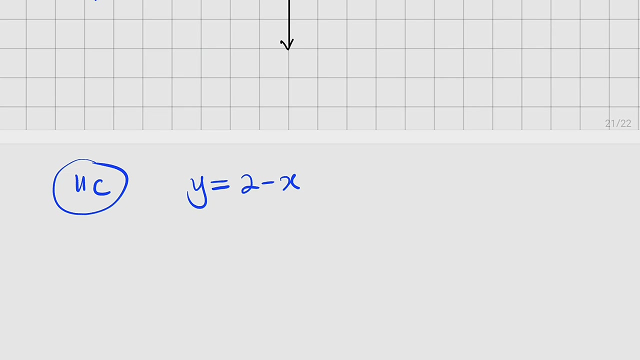 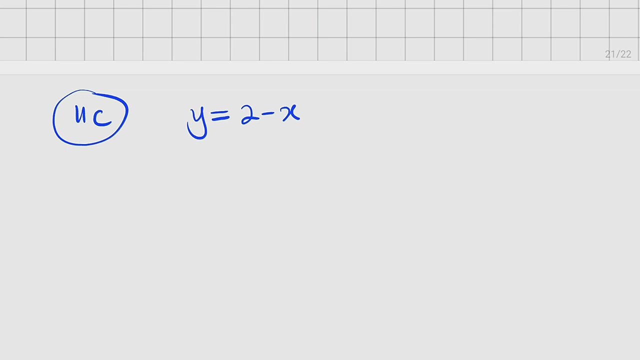 So 11c, the equation is y equal to 2 minus x, right, But let me confirm: Yes, 2 minus x. You know, only two points are enough for you to construct a straight line graph. So we are going to form x, y, 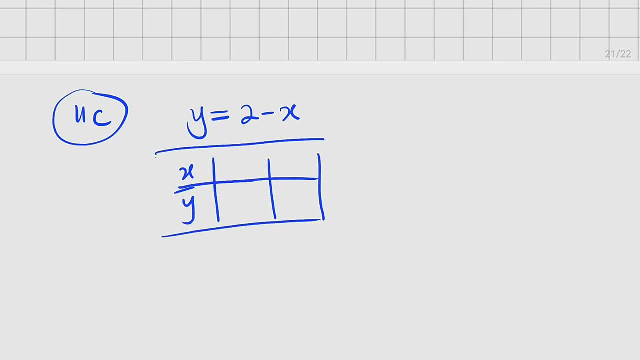 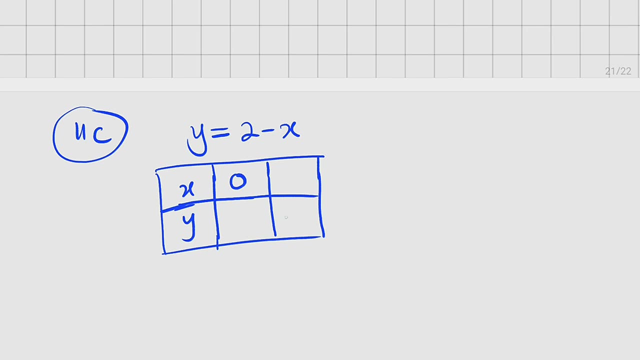 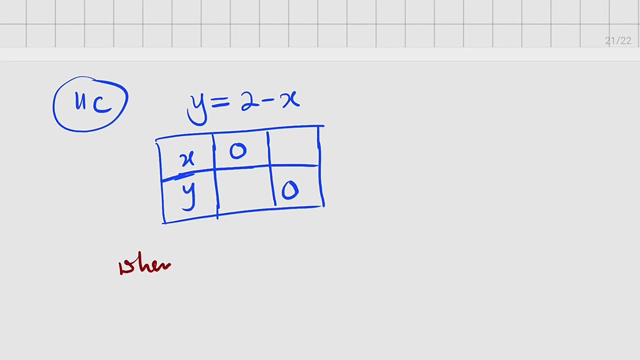 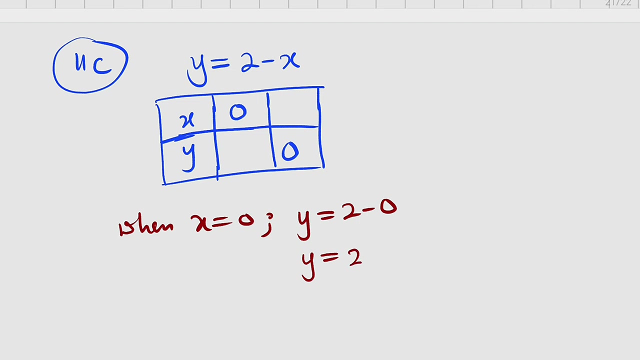 This is a table. So what will be the value of y when x is 0? And also what will be the value of x when y is 0?? These are only things we are looking for. So when x is 0, we have y equal to 2 minus 0, which implies that y is equal to 2, right. 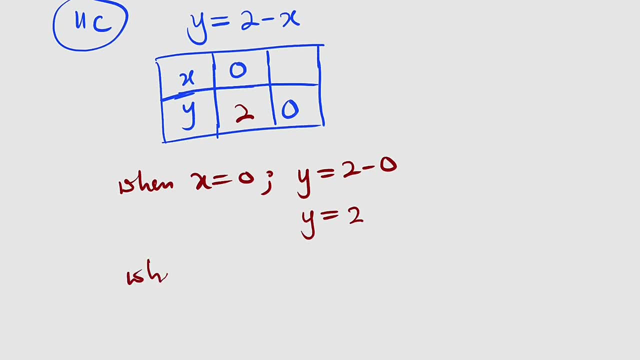 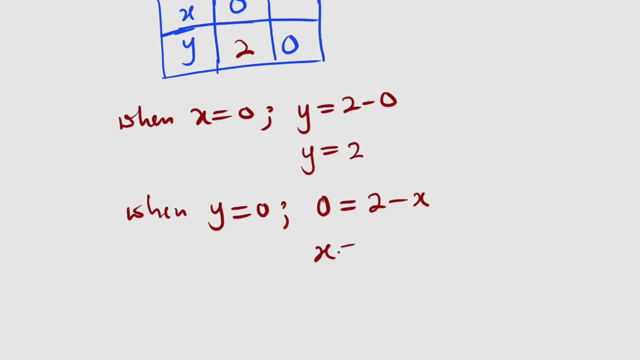 Then you write 2 here. But when y is equal to 0, what happens? We have 0 equal to 2 minus And x. Therefore x must be equal to 2.. So you write 2 here. So these are the two points we need. 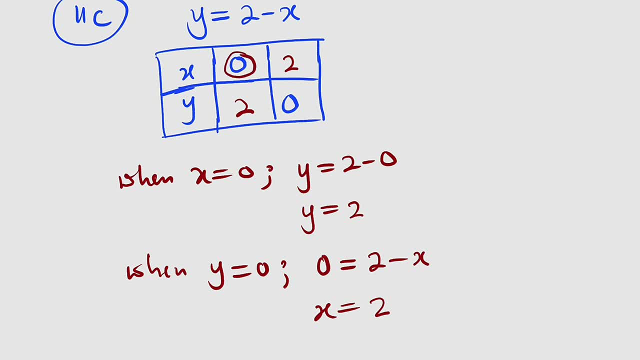 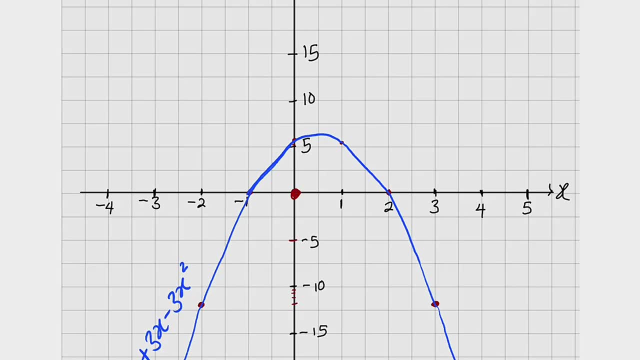 On the graph we are going to locate where x is equal to 0, y equal to 2.. Let me start with this point. This is where x is equal to 0. But we need to find out where y is equal to 2.. 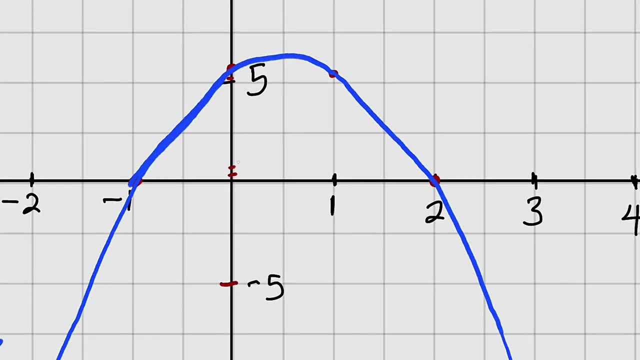 Remember, I told you we have five lines here: 1., 2., 3. 4. 5.. So y will be 1 here, It will be 2 here, right? So this is exactly where it is equal to 2.. 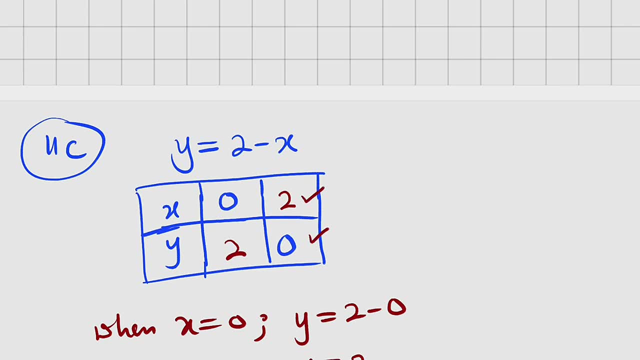 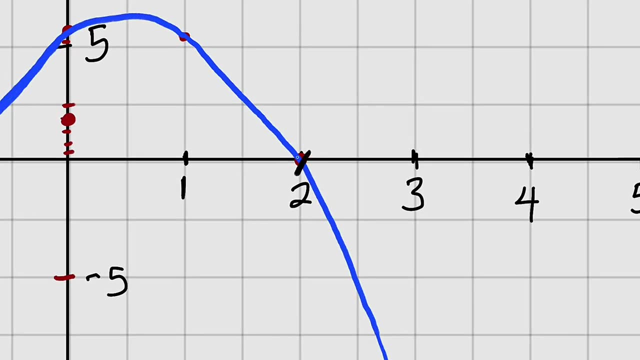 Then we look for where x is 2, but y is 0. This is where x is 2 and y is 0. So let's have a star here. So what do we need? We need to use our ruler: connect these two points together. 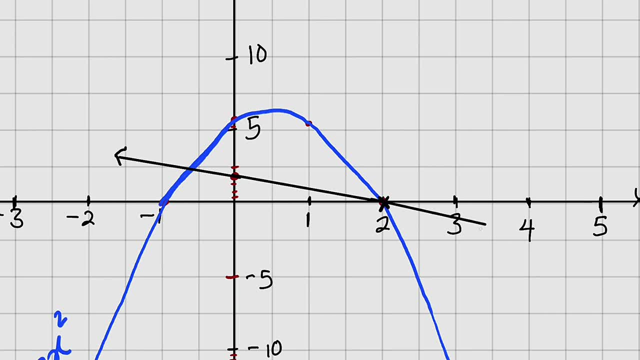 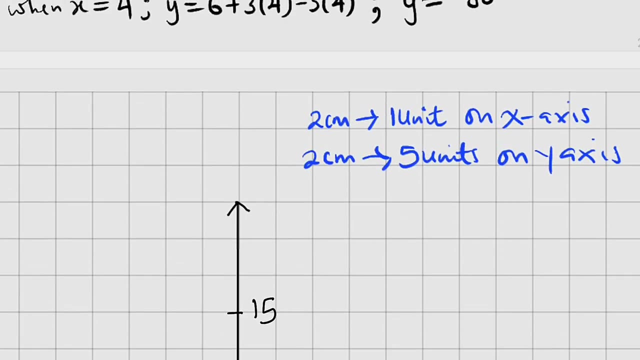 All right, you can see this is the graph of that function. So let me name the graph. We can name it as y equal to 2 minus x, So both b and c part are all done in the same graph. So now let us look at the next question. 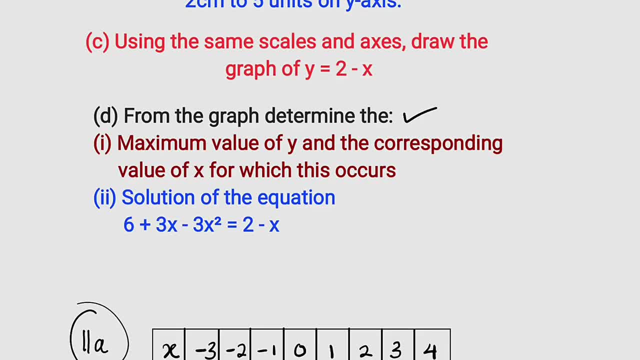 Then the d part. it stated that from the g part, from the graph, we should determine the maximum value of y. We are referring to the first graph we have constructed. The maximum is exactly where the parabola takes a turn. So we want to find the value of x and y at that point. 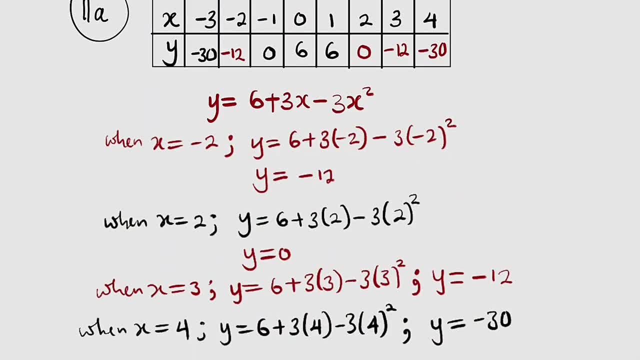 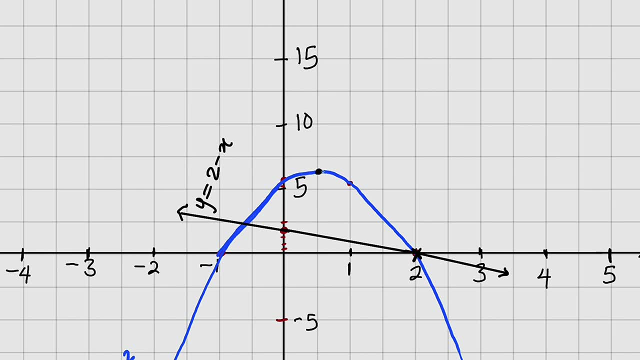 And that is the first question, before we come back to this one. This is exactly where the parabola takes a turn, and that is the maximum value it can take. You see, the value of x at that point will be 0.5, right. 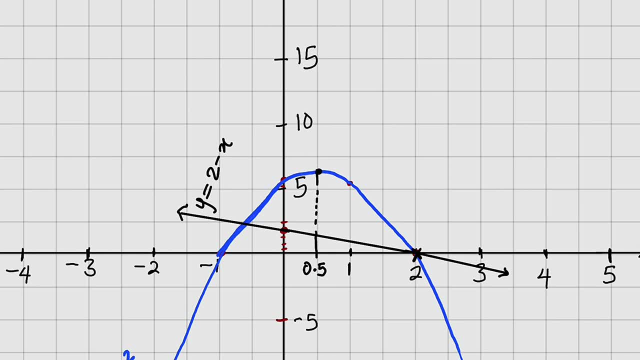 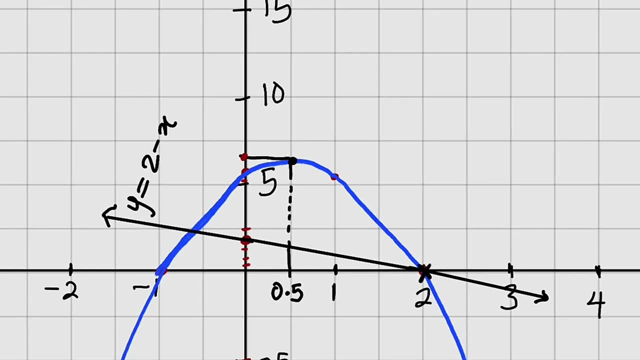 This is 0.5.. So now let us find the corresponding value of y. You have to come to this direction. This is exactly the corresponding value of y, So let's estimate it here: 1,, 2,, 3,, 4.. 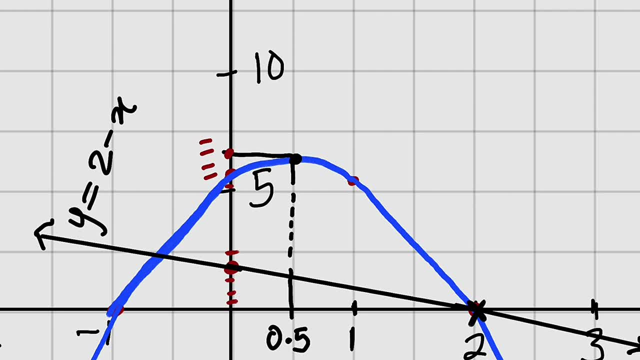 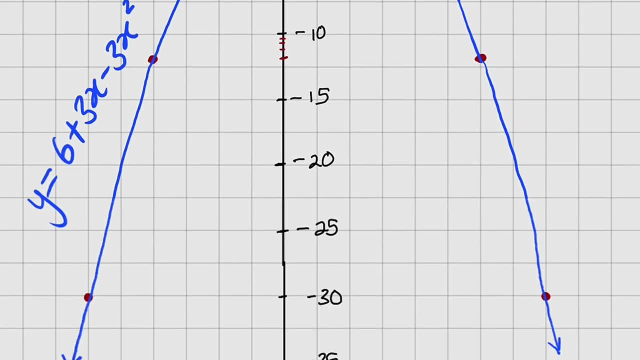 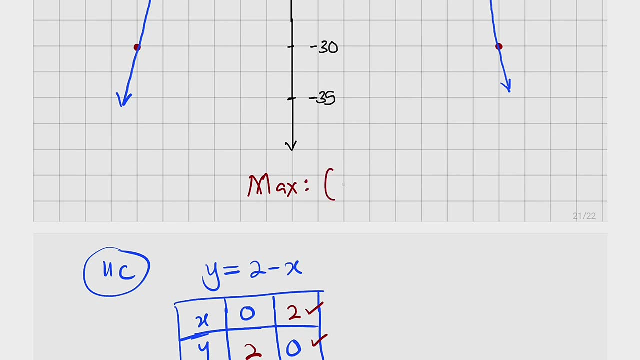 So it will be 6.5, approximately. So this is 6.5.. So you can do it down here. The maximum you can write it here. Max is at when x is 0.5, y equal to 6.5.. 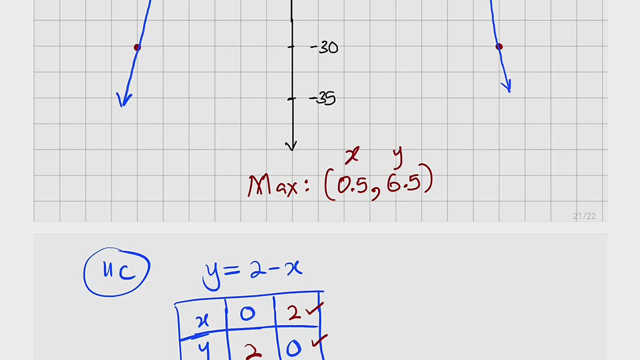 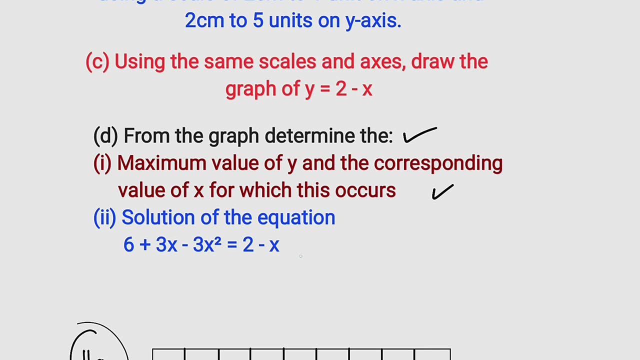 This is the maximum where this is for x and this is for y. Now let us move on to the second part. The second part. we are asked to find the solution to 6 plus 3x minus 3x squared. We are asked to find the solution to 6 plus 3x minus 3x squared. 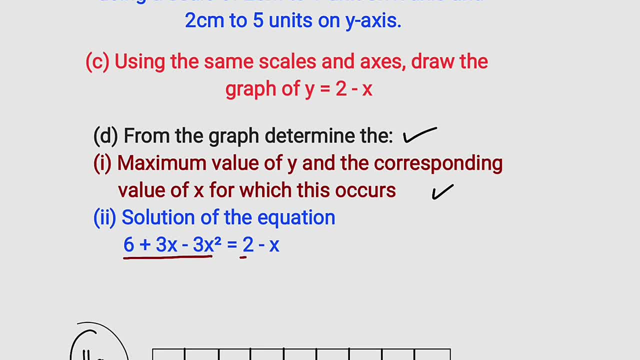 Remember, this is the parabola we have constructed and this is the linear graph, which is the straight line graph. If we want to find the solution on the graph, we are going to determine those two points where the two graphs intersected. 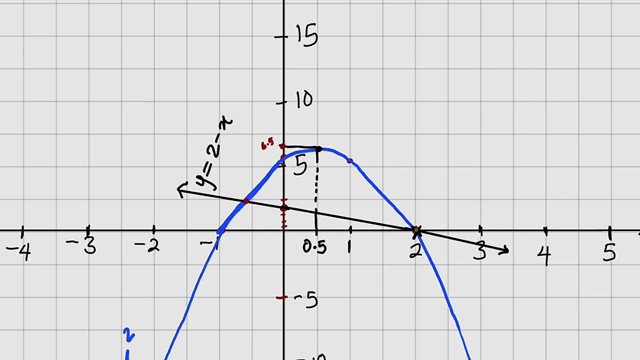 So you can see they have intersected at this point and also at this point. So what is the corresponding values of x at that point? And that's said to be the solution to the problem. So if you come down right here, we are going to have approximately 0.6 here. 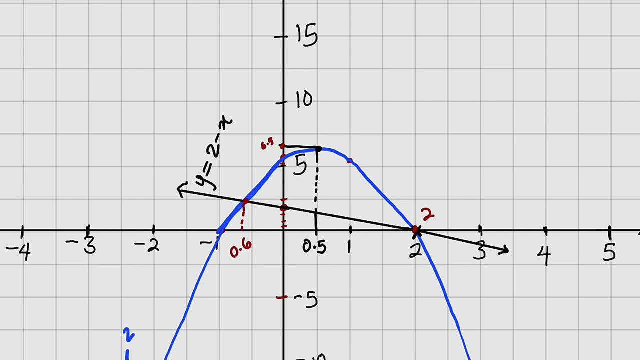 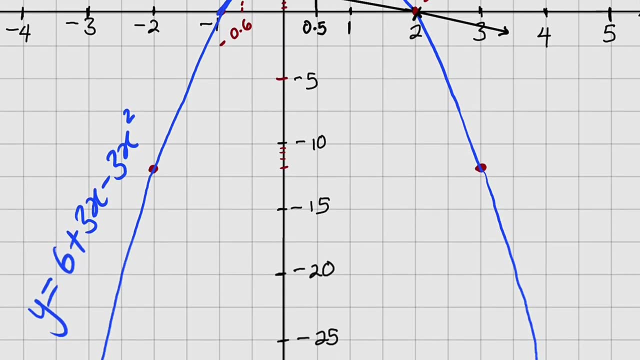 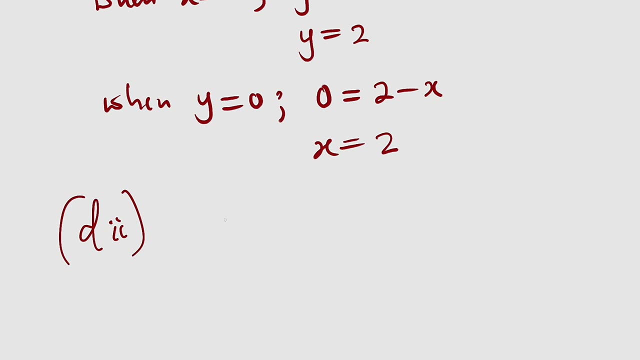 and you can see this is 2.. So the solution to the problem is either 2 or negative 0.6.. So the d part, the d part which is Roman, 2, 6 plus 3x minus 3x.